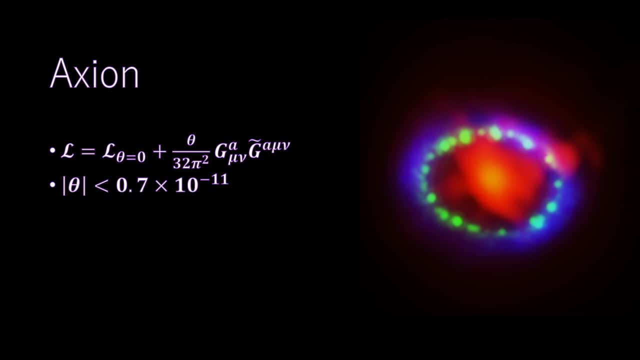 violation is determined by an arbitrary parameter, theta. however, the magnitude of theta is restricted by experiments measuring the electric dipole of neutrons and is known to be almost zero. it is natural that all terms that have no reason to be prohibited appear, so the cp conservation in 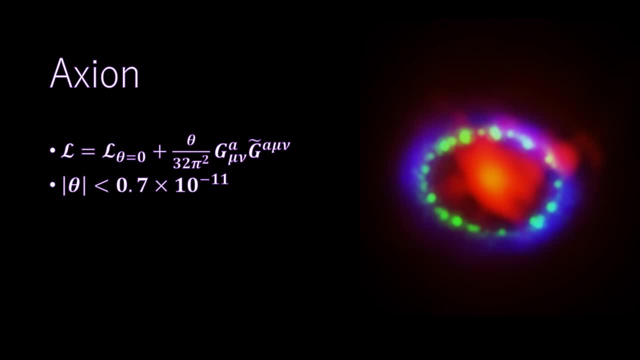 qcd means that qcd is an unnatural theory. rd pecky i and r quinn have worked out a solution to this issue. they introduced a new symmetry called pecky i- quinn- pq symmetry regarded theta as a scalar field and obtained theta equals zero as the solution with the minimum potential in this model. 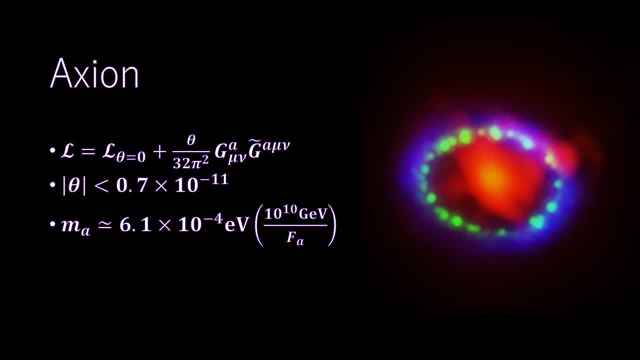 the pq symmetry breaks the pq symmetry and the pq symmetry breaks the pq symmetry and the pq symmetry at a certain scale of energy f, which produces scalar particles known as nambu goldstone bosons. these scalar particles are axions. action gains mass m through the instanton effect of the qcd. 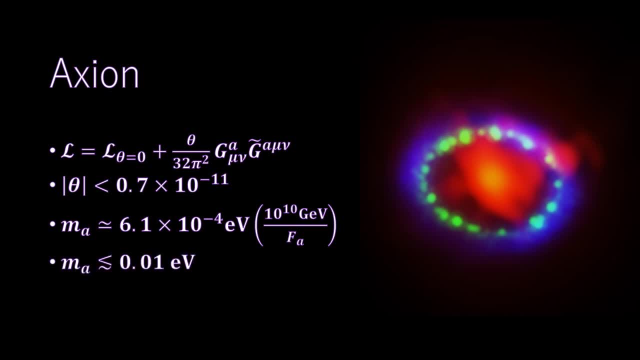 the existence of the action has not yet been verified experimentally, but the mass of the axon is severely constrained by ground experiments and the analysis of astronomical phenomena. since the strength of the interaction between the action and other particles is proportional to the action mass, the upper limit of m can be obtained the most. 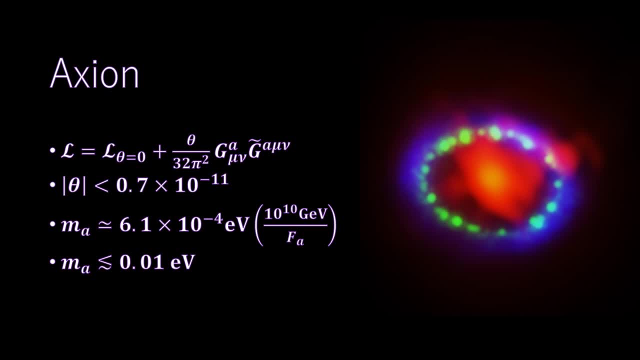 stringent restrictions are achieved by supernova sn 1987a. axions with a large f interact only very weakly with other substances. therefore, when an action is created in the core of a supernova, the energy can be taken out of the supernova and the supernova cooling is accelerated. 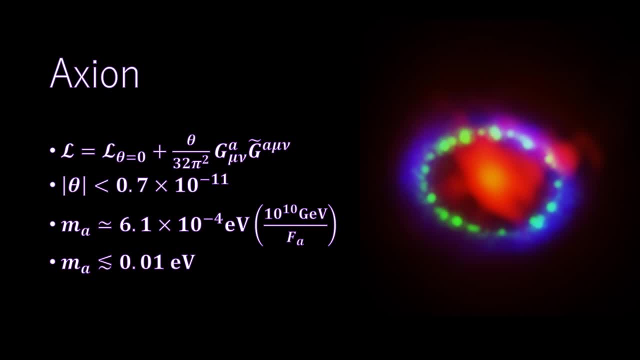 when the action cooling is effective, the energy that neutrinos bring out of the core is reduced, which contradicts the observations of neutrinos emitted from SN 1987a, resulting in the strong limitation. If there are many light axions in the universe, it can be dark matter. The supersymmetric theory has favorable features. 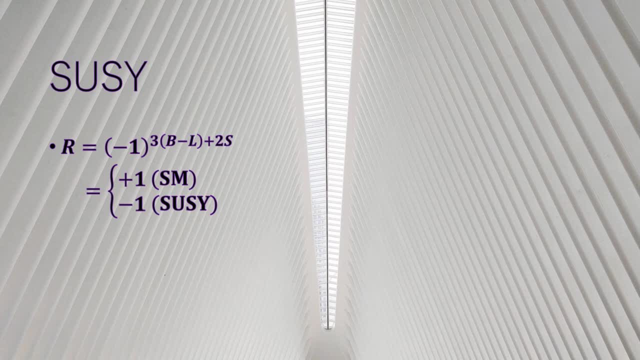 such as solving the hierarchy problem and realizing unification of coupling constants in guts. The supersymmetric theory requires a symmetry commonly referred to as R-parity. Here, B, L and S represent the baryon number, the lepton number and the spin respectively.